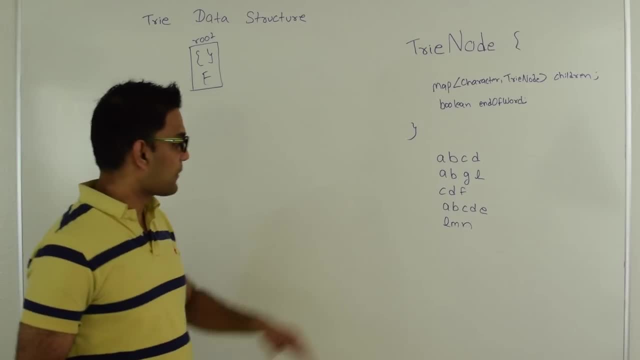 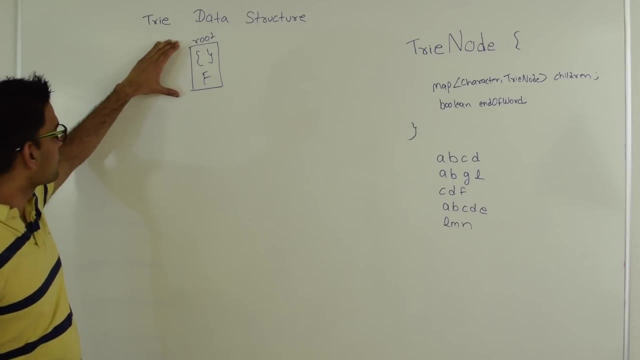 example, unicode character set. So next, what I'm going to do is I'm going to insert this five words into a try. So initially the try, our try, is a root and root has an empty map. so this map here is empty and then boolean end of word is false. So then 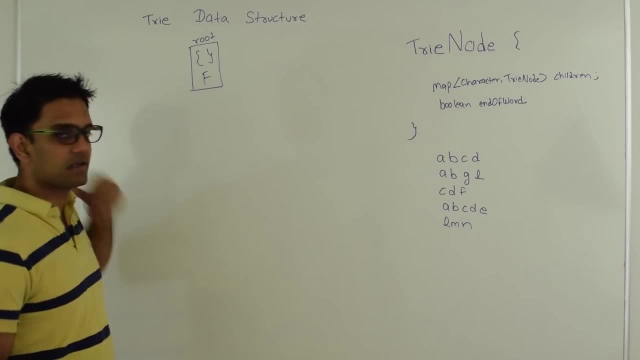 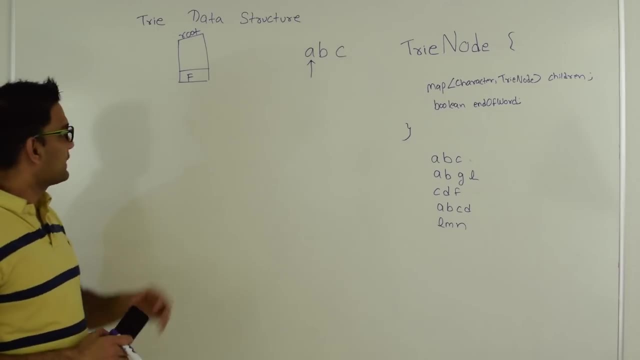 we're going to take this word abcd and insert into this try. So our index is pointing to a and we are at the root of this try node. So first we check is: does a is a present in the map of this root? So map of the root was empty, so a is not. 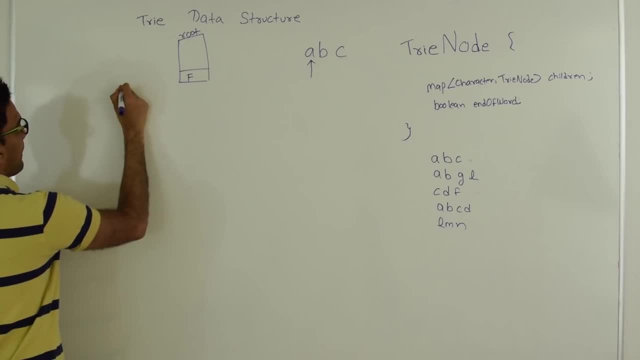 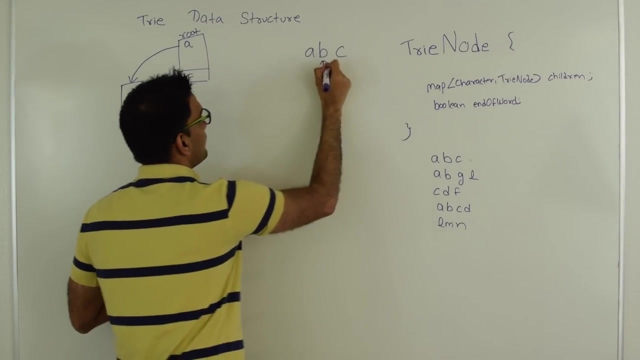 present. So then we create a new try node whose end of word is false, So this boolean is false for this try node. and then we put a into this roots map and for the value we put the reference of this newly created try node. So effectively we are creating a relationship like this. Then we increment this to b and: 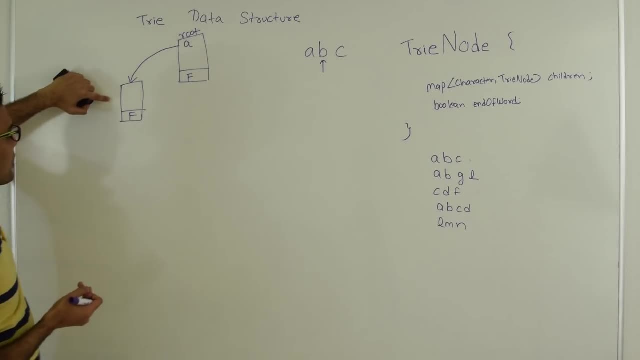 then we move here. So here we check: does b belong? is b present in this try node, in the map of this try node? So again, since this was newly created, b is not present. So we create another try node with the value false- end of word, value false- and put b in. 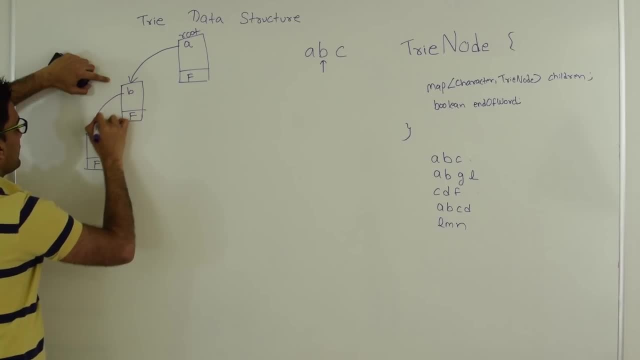 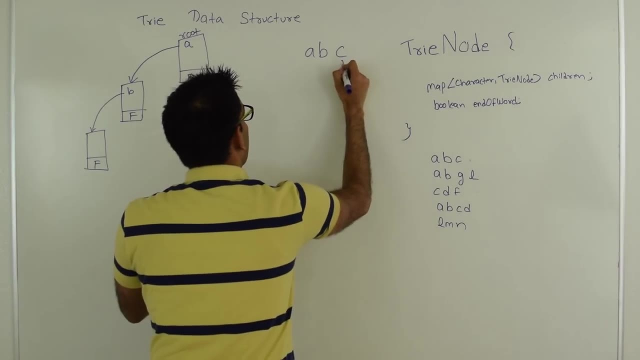 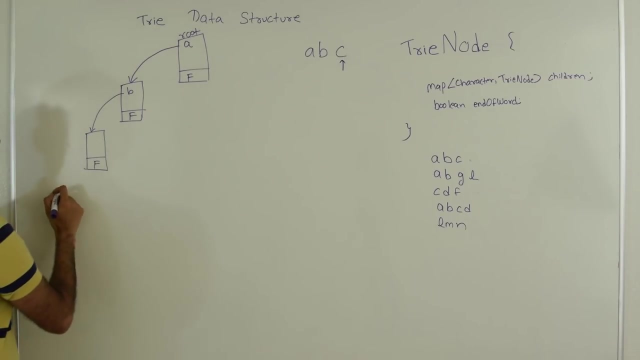 the map of this try node and point it to here. and then we move here and we increment this guy to c. So does c exist here? So again, this was a newly created try node, so its map is empty. so c does not exist. So we create c. 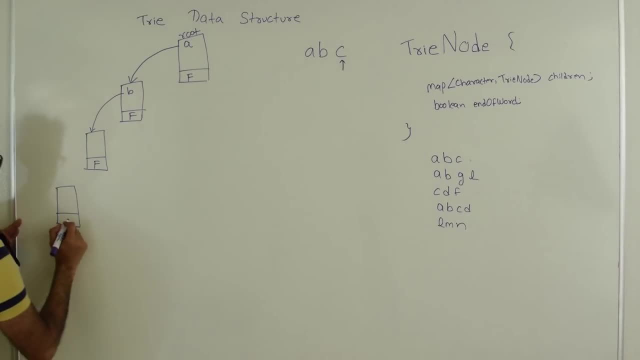 And since c is the last character of this word, in this case this value here will be true. And then we are going to put c in the map of this try node and point it to and point the reference to this try node. So this is how we inserted a, b, c into an: 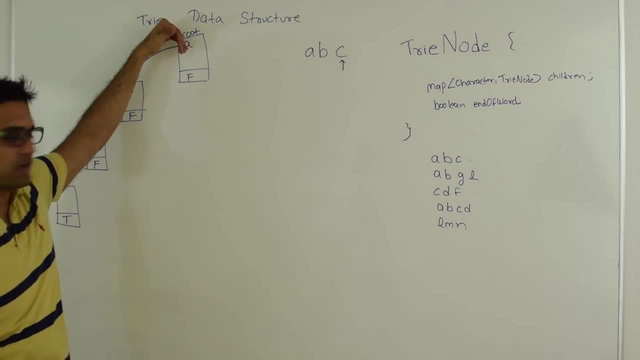 empty try. So all we did was we started with root, put a in there, then we went to b, put to this guy, put b there, then we went to this here and put c there and then finally we reached here and since this was the last, this was the last, this represents the last character. 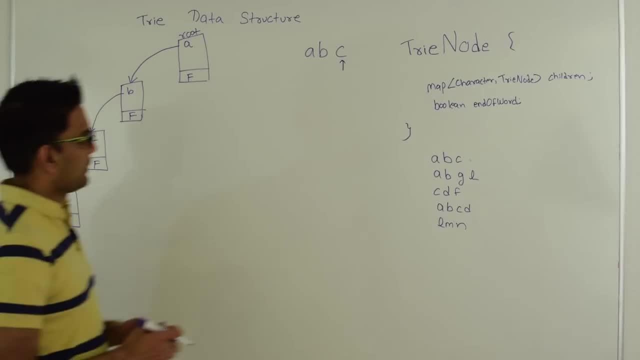 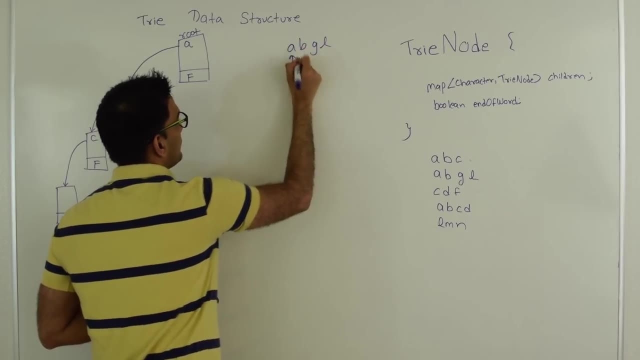 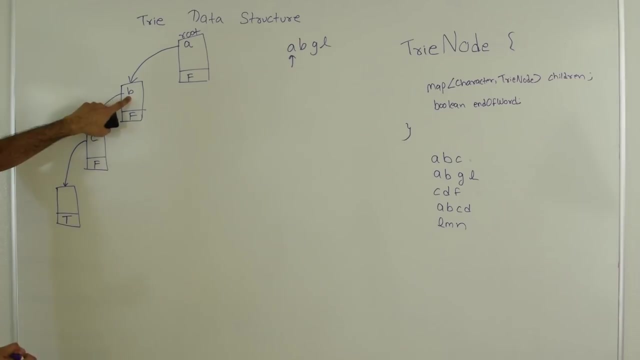 of this word. we mark this end of word as true. So next let's try to insert this word: abgm. So again we start with a and we start at root. Does root have a? So root does have a, So we jump here. Does this trinode have b? So this trinode does have b. So we jump here. 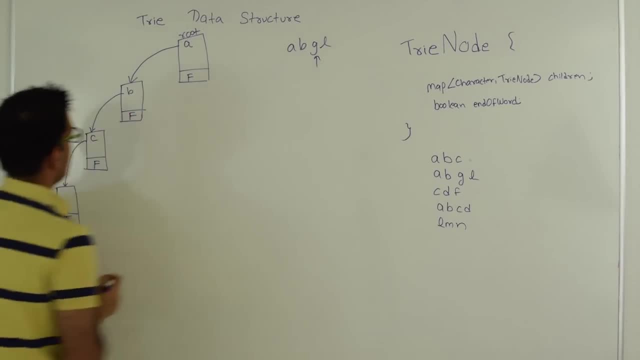 and our pointer is now at g. So does this trinode have g? It does not have g, So we're able to create a new trinode whose end of word is false It's. and then we put g into the map and the reference of this in the value of the map here. 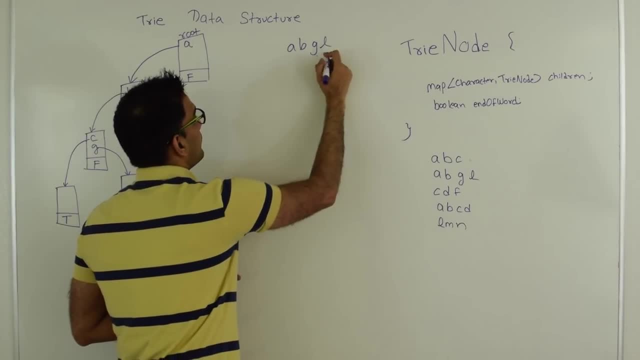 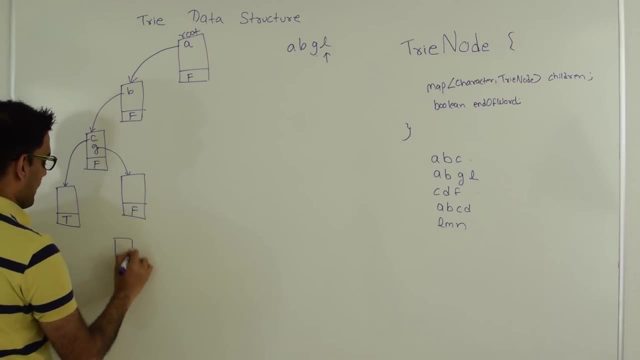 And then we move one more. So this comes to l. Does l exist here? L does not exist here. So we are going to again create a new trinode and since this is the last character of this word, this value will be true, and we're going to put l here and point this way. So now we 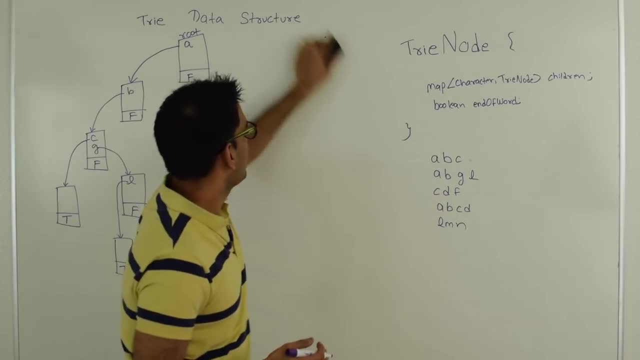 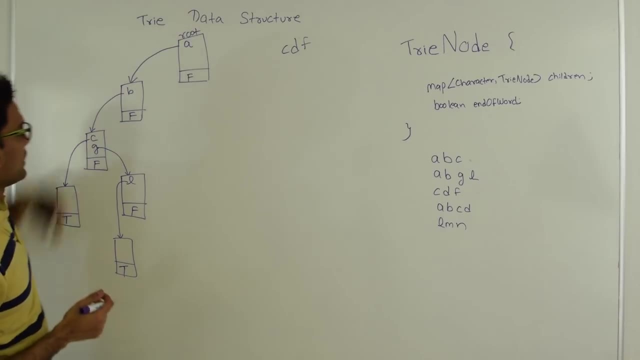 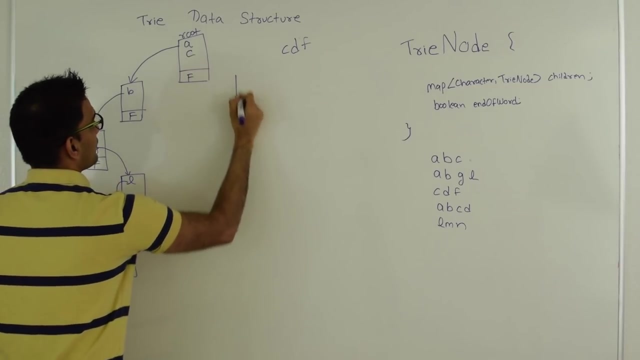 are done, inserting abgl. So next let's try to insert cdf. So again we start at root. Does root have c? So root does not have c. So what I'm going to do is I'm going to insert c, create a new trinode whose end of word is false and point. 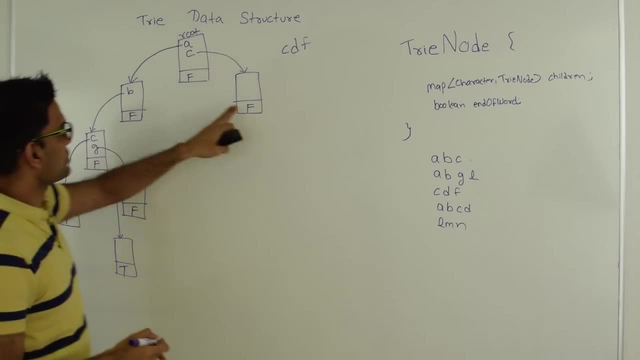 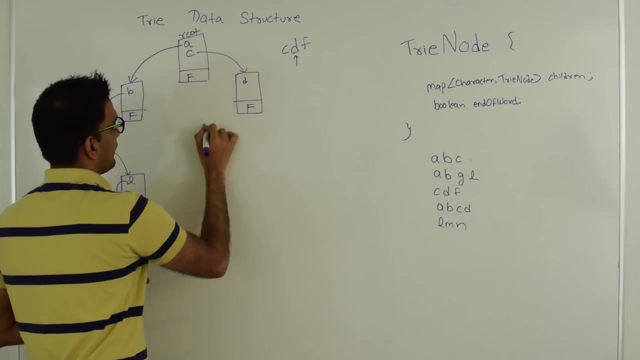 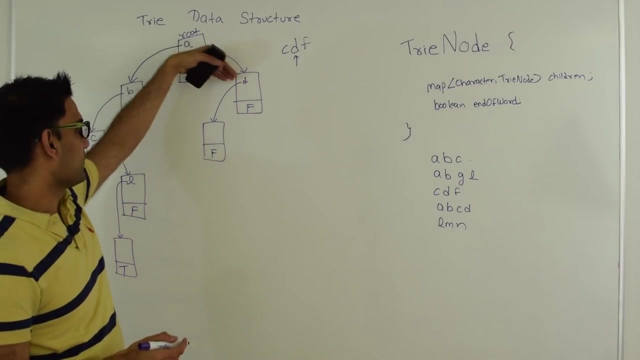 this here. And then we jump here and our index is now at d. Does this guy has d? It does not have d. So we create a new trinode with the value false and point this to d And point the, put it in the map d and the reference of this trinode, And then move to f. So f. 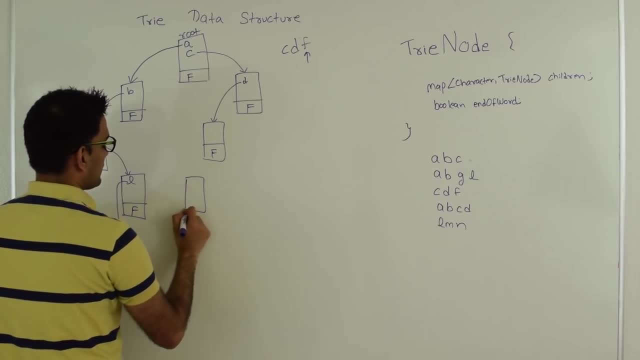 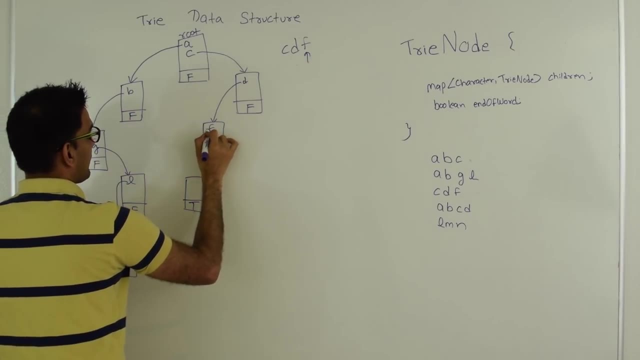 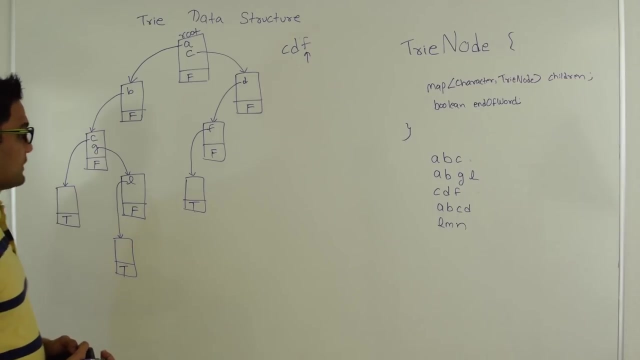 does not exist here, So I'm going to create a new trinode. Its value will again be true, because this is the last character of this word and we'll say that f points this way. So finally, we are done inserting cdf. Next let's try to insert abcd. So again we start. 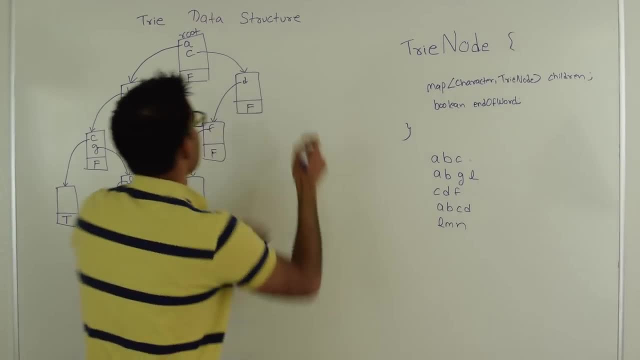 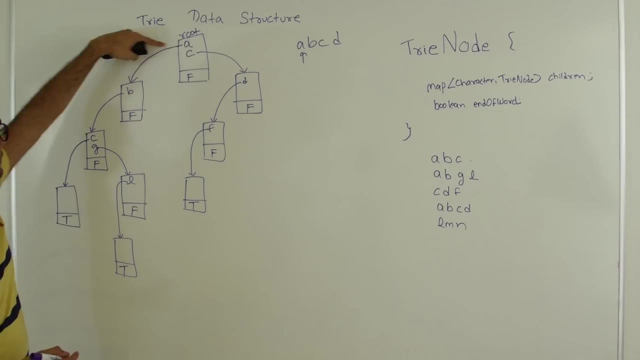 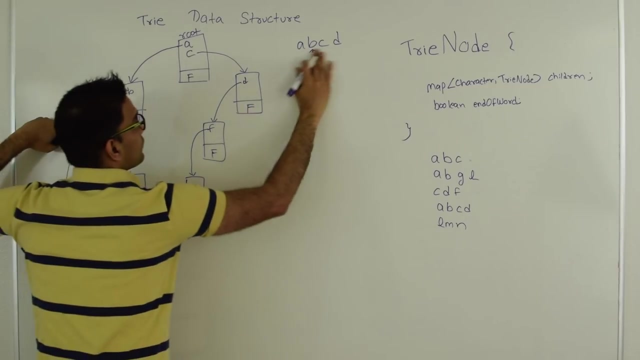 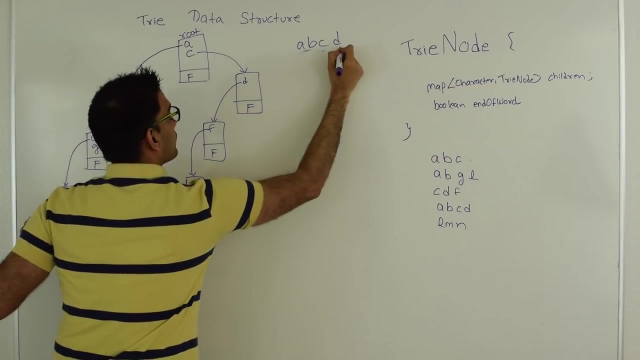 from root. Again. we start with root. a is there, so we follow the pointer of a and reach here, So here. b is also there, so we follow the pointer and reach c, So c is also there. so we follow the pointer and reach this point And in here. so now our pointer is pointing: 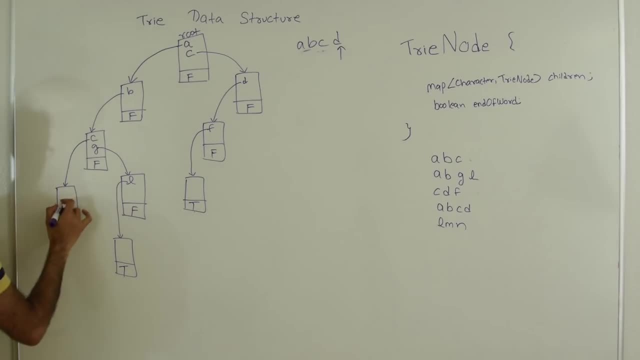 to d. So here d does not exist. So what we're going to do is we're going to add d here, So add d, create a new, create a new trinode. Since it's a last character, mark this as true. Add d and reference of this guy in the map here. And this is how we add it: d. 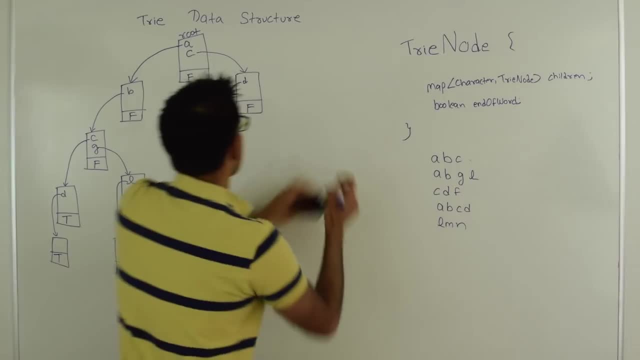 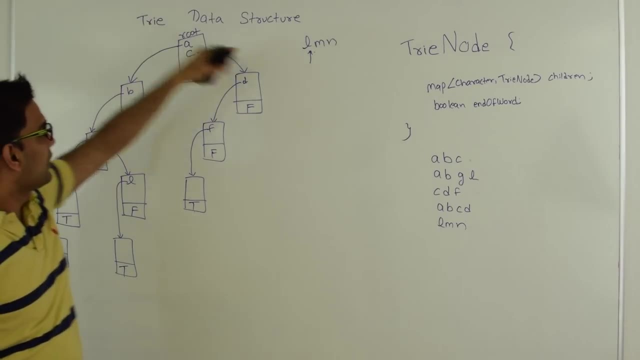 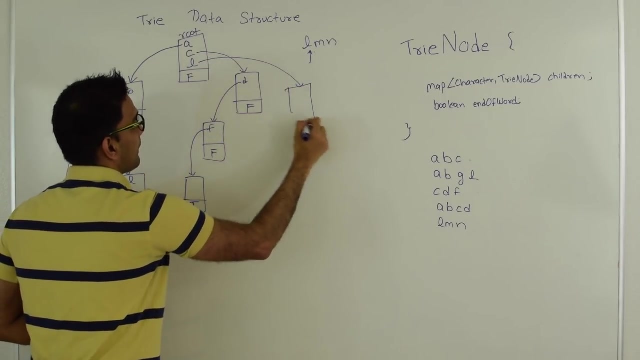 Finally, let's add this word, lmnn. So our root. again. we'll come back to root. lmnn is the last character of this word. So here d does not exist. so we're going to add l and we're going to create a new trinode for l with the value false. and then we move. here m does not exist. 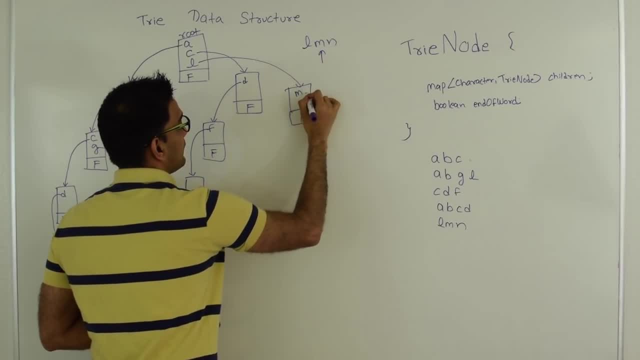 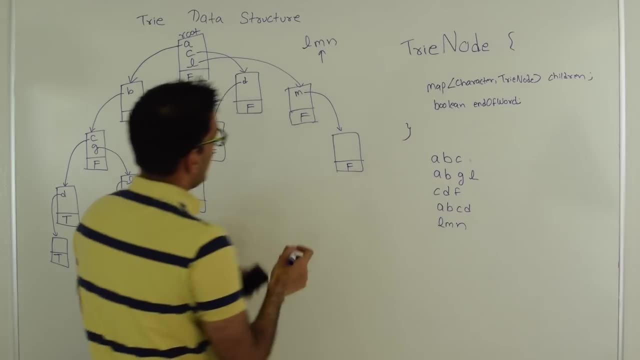 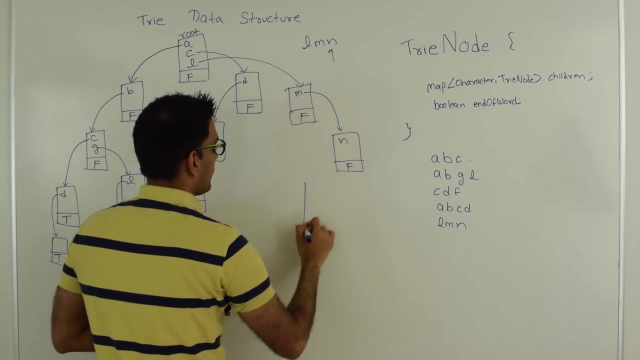 so we're going to add m and follow the trinode here- false- and then we move this to n and n does not exist here. so we're going to create n And follow this trinode and n jumps here. And since this is the last, n is the last. 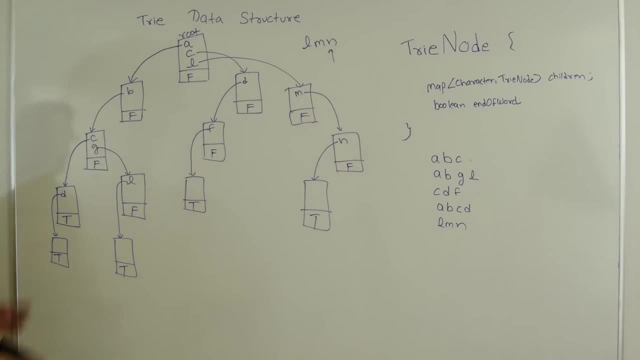 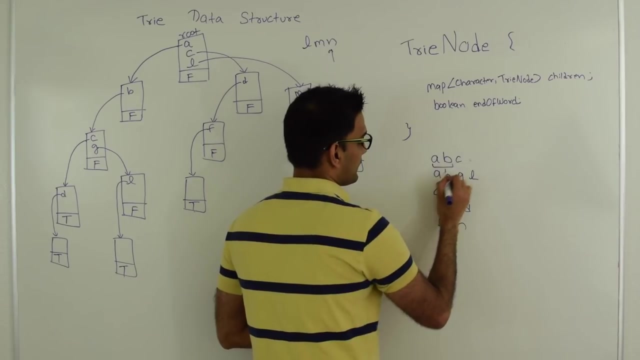 character, this value becomes true. So this is how my trine looks after I'm done inserting all this five, five words in my trine. So, as you can see, if two words have the same prefix, so for example this and this, in this case they share the common ancestors, So this: 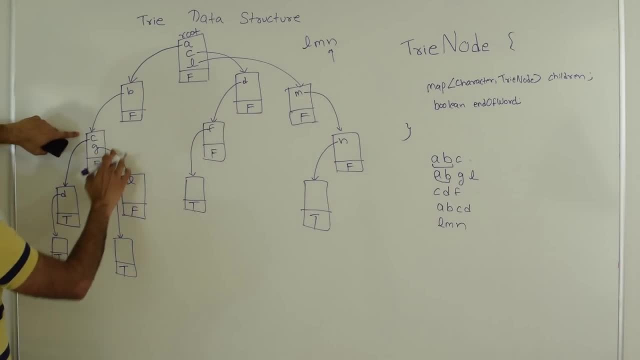 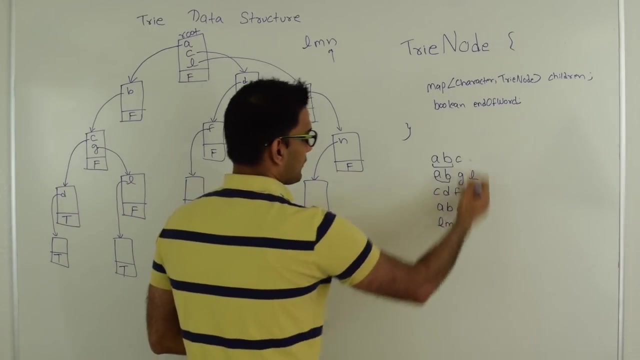 here abc and abgl. so they have same, they have same prefix, so they share this common ancestors and from this point they bifurcate. So the time complexity for this is pretty straightforward to see If the average length of the word is l and total number of words: 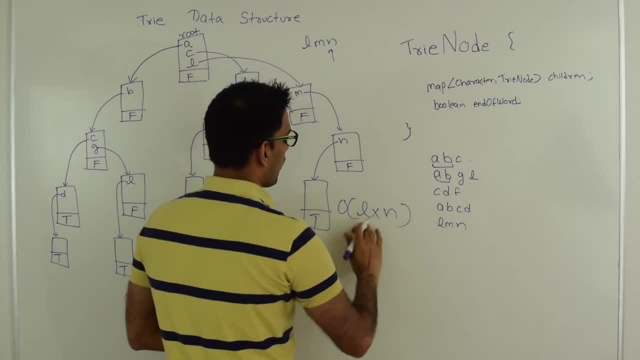 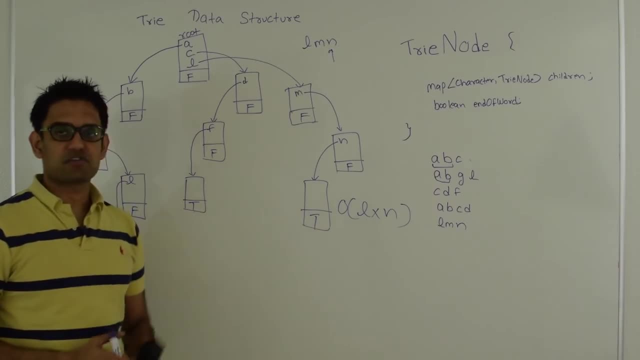 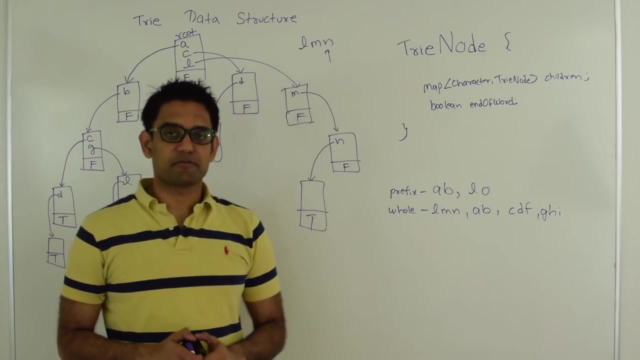 are n, then the time complexity is o of l into m. So next let's look at how we're going to do a search in this Try. There are two kinds of searches: Prefix based search, where we're checking if there is at least one word which starts with a given prefix or not, and then the whole word search. 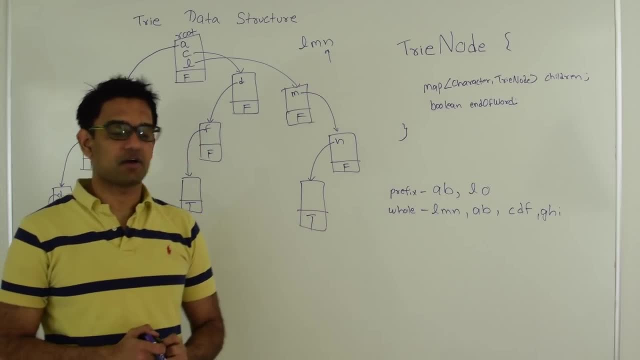 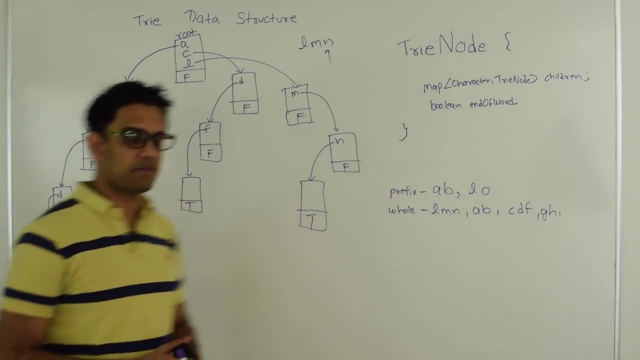 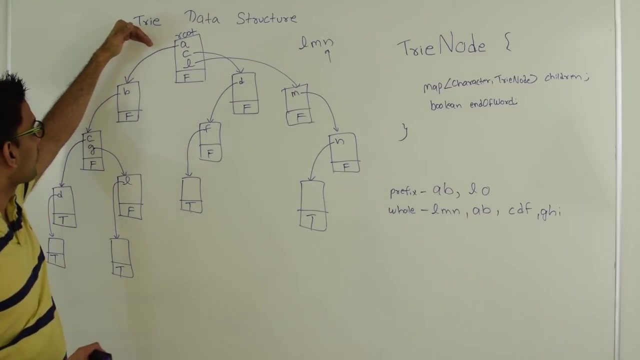 where we're checking if the entire word exists in the try or not. So let's start with a prefix based search and see if there is any string in this try which starts with ab. So we are at root. we check if the map, if this map at the root, contains a or not, So it does. 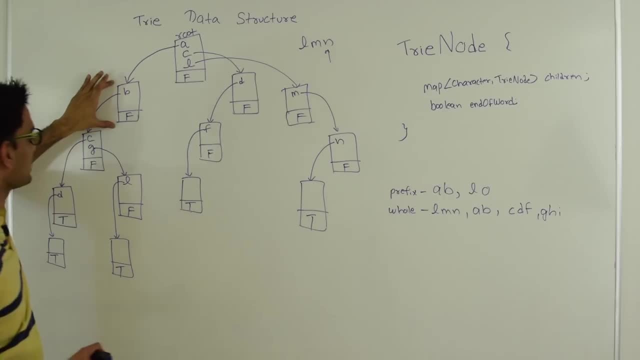 contain a. so we jump to that trinode, So we reach here, Then here we check if the map in this trinode contains b or not. So it does contain b. So what this means is there is at least one word which does start with. 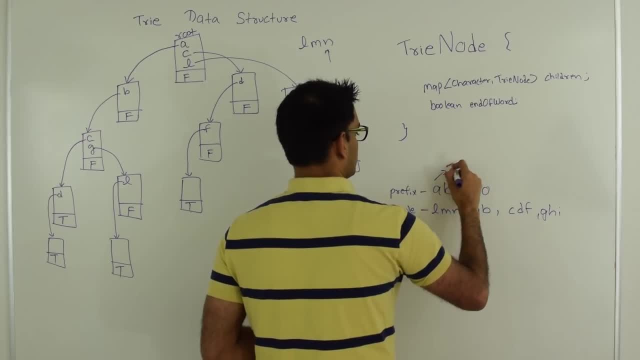 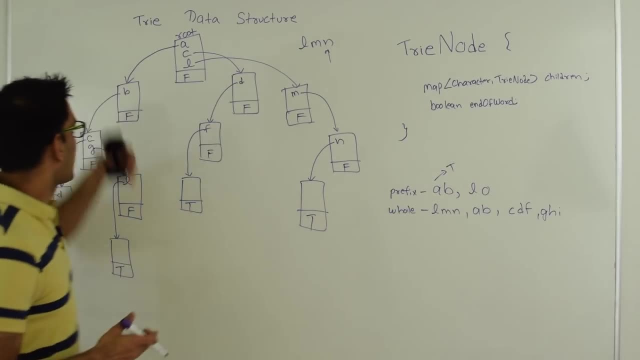 ab. So this should return true. There is no reason to look forward into this try. Let's look at lo. So again, we start at root. we check: is there, does l exist in the map of the root or not? So l does exist. so we follow its trinode and reach here. Then we check: does o exist in? 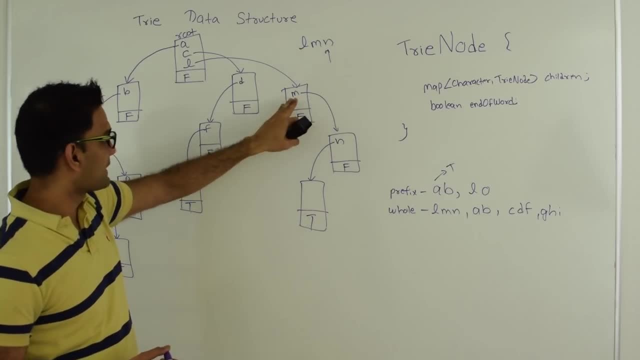 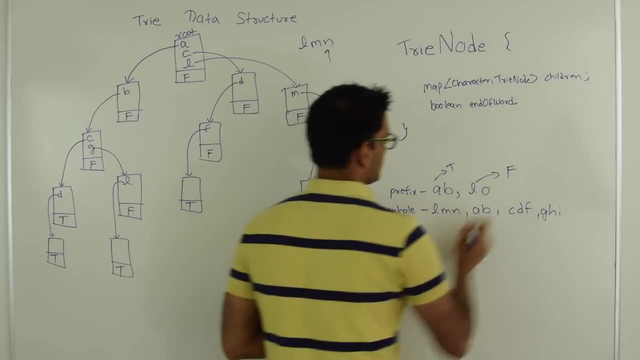 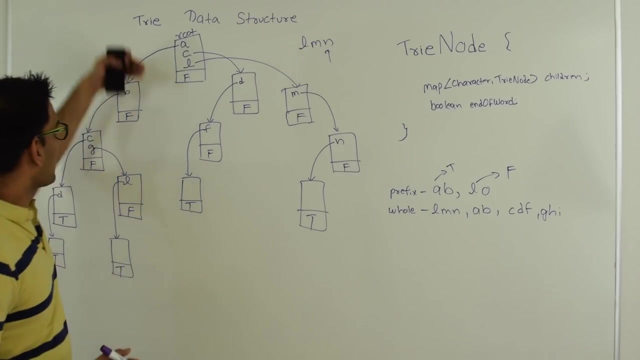 this trinode or not. So ao does not exist here. So what that means is there is no word which starts with prefix lo, So this should return false. Let's try some whole word search. So let's try and start with l and n. So again we are at root. we check: does root have l? 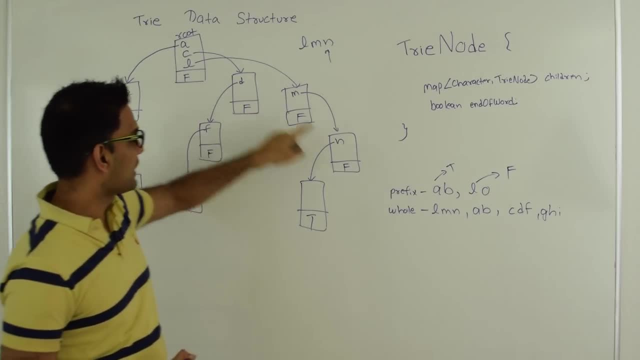 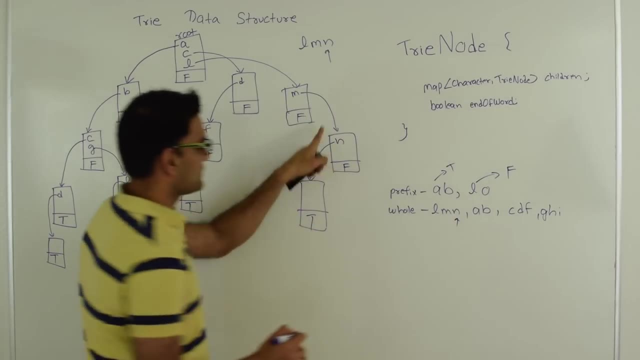 So it does have l. so we follow here. Then we check: does this trinode have m? So it does have m. so we follow here. And then we check: does this trinode have m? So it does have n. so we follow here and reach this point. 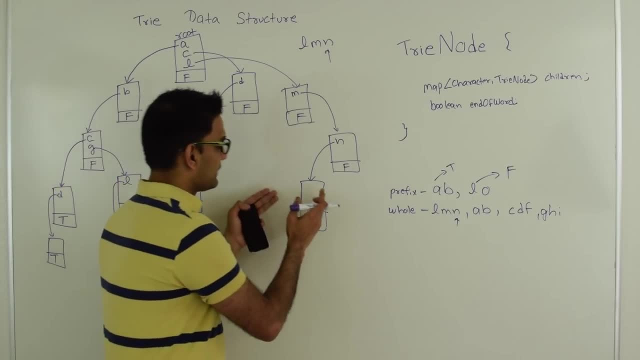 Once we reach this point we check: is this node? is the end of word value here true or not? And that is very important. So end of word here is true. It means that l, m and n does exist in this try, So this should return true. 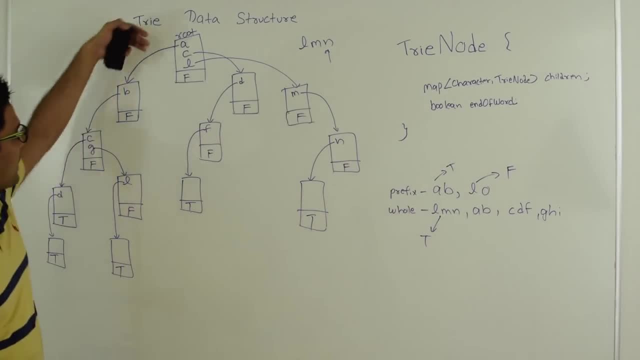 Let's do ab. So again, we start at root. we check a exists or not, So a does exist. so we follow here. Then we are here and we check if b exists in this trinode or not. It does exist, and we follow here. And now we look at the value here. So this value, end of word. 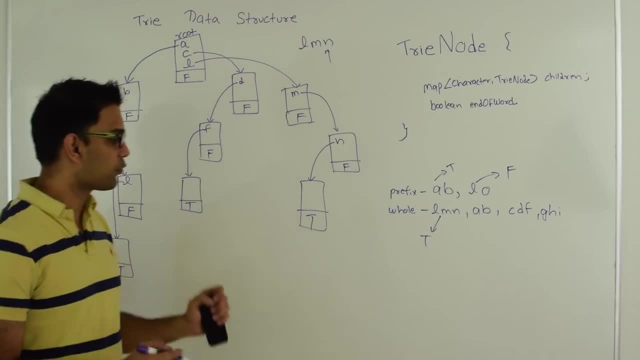 is false. It means that there is no entire word ab in this try, So this should return false. What about cdf? So we are at root: Does c exist? It does, So we move to. we move it follow its pointer. 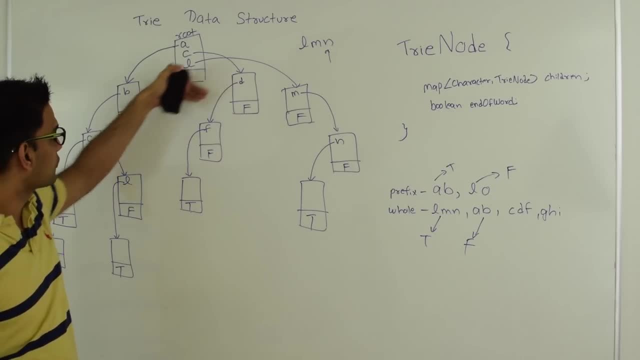 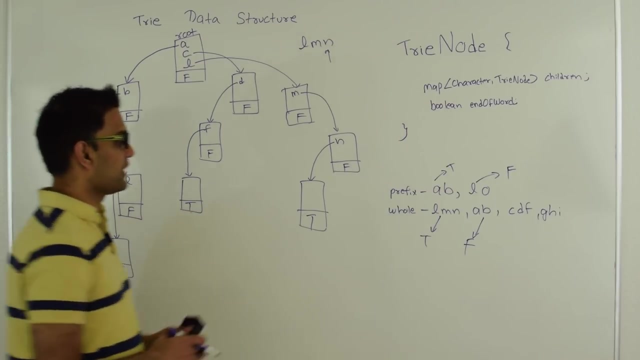 reach d. Does d exist? It does. So we follow its pointer: reach f. Reach this node. Does f exist in this node? It does exist. so we follow this pointer and reach here. And then the end of word is true. It means that cdf does exist. And finally, ghr Does g exist. 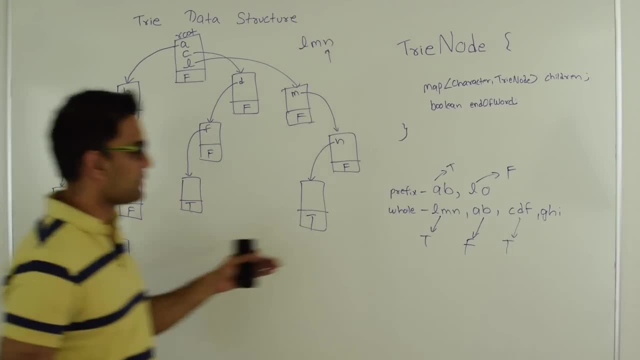 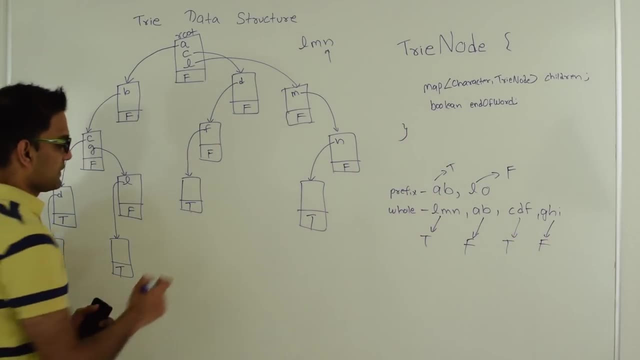 in the root node. G does not exist in the root node, which means that word ghi does not exist. So this should return false. So again, the time complexity is very simple. If the length of the word is l, then the time to search will be o of l. Next let's look at 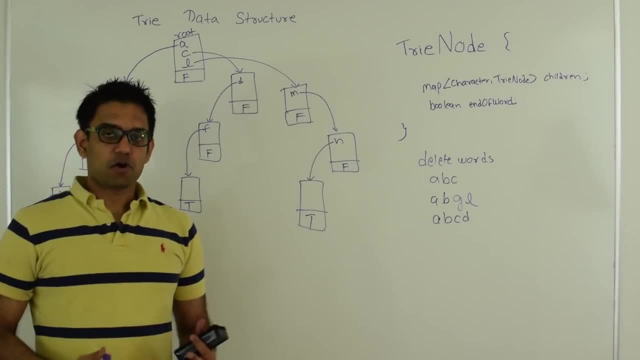 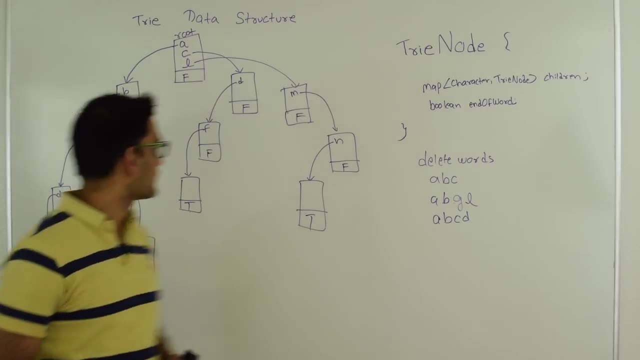 how we are going to delete in this try. So delete also exists in two flavors. One is delete the entire word, or second is delete all the words which start with the given prefix. So we are going to try to delete this word. abc. We are at root. A exists here. we follow. 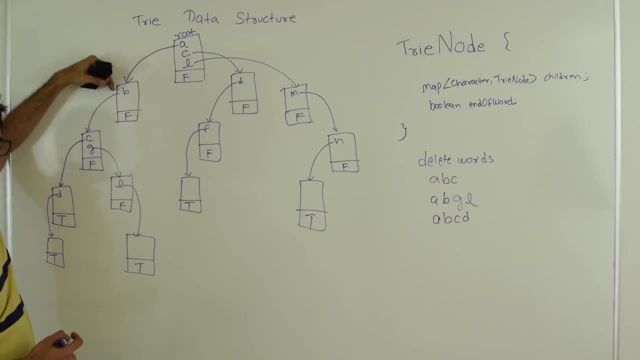 the link. reach this point. this try node B exists here. follow the link. reach this. try node C exists here. follow the link and reach this try node. So now we have to delete this word abc and we are here. So the thing is, we cannot just delete this node. Why? 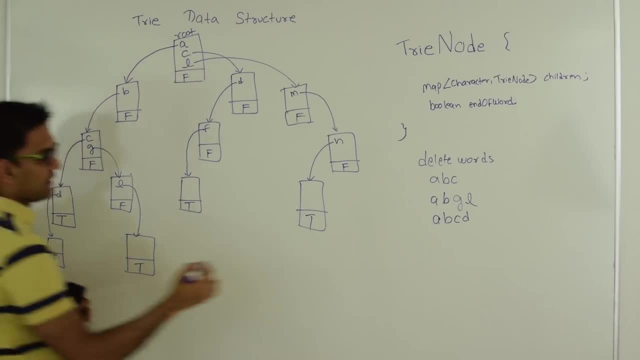 Because if we remove this node from this try node, then in that case we would also lose the word abcd, which is repetitive, Presented by this link here. So what we do is, since the map at this try node is not empty, we cannot get rid of this node, So all we do is turn this into false, Turn this end. 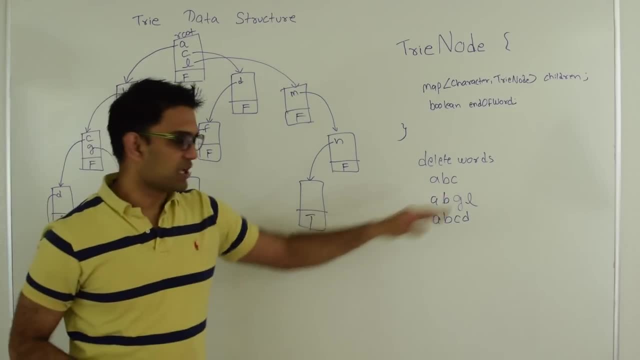 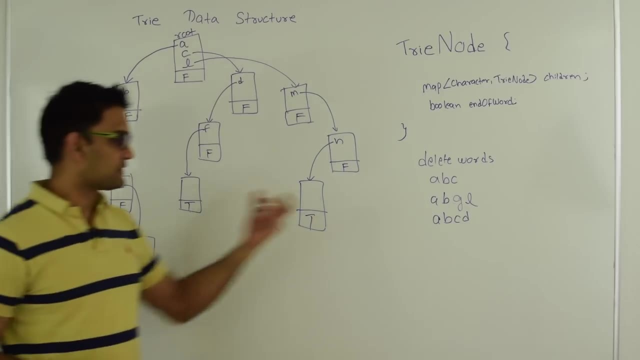 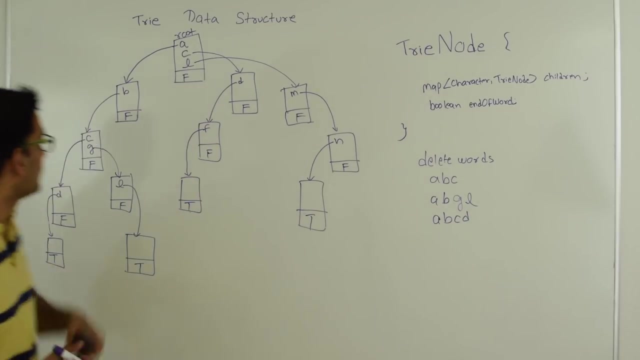 of word into false. So now, if someone searched abc, he would reach this point and since this value is end of word- is false, then they would say that abc does not exist in this try, and that's how we deleted abc. Next we will try to delete abg out. So we start with root. follow link: reach this try. 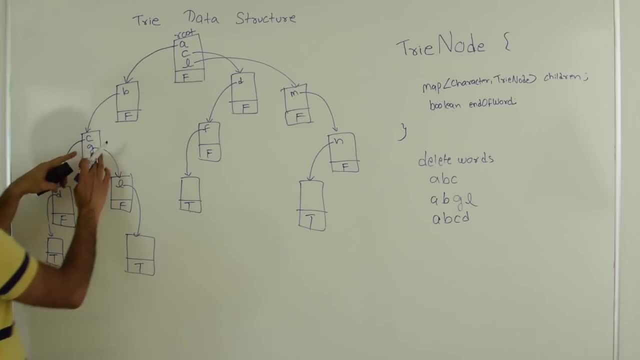 node, follow link, reach this try node. and then from here we follow this g link and reach this try node. and then from here we follow this l link and reach this try node. This try node has no children. Why? Because its map is empty. So then we can safely delete. 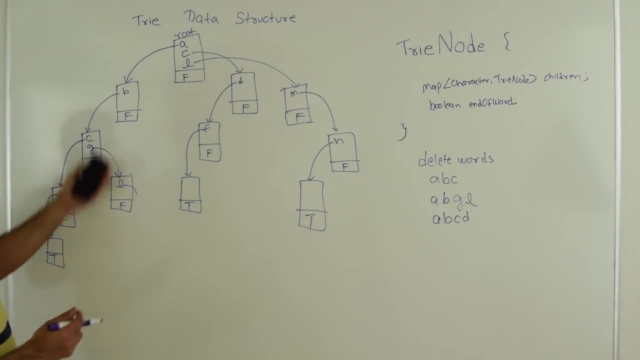 this guy and then try to delete the nodes at the higher level too. So now that this is deleted, we can remove this character from its map, and as soon as we remove this character now, this map is empty. so we can delete this as well and go one level. 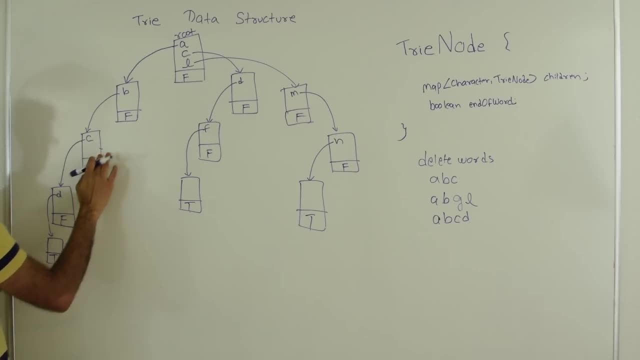 up here and delete this value g. Now we cannot delete this node because this has another link. This also has c, So at this point we will stop. So we are done deleting abg out. Next we will delete abcd. We follow abcd and we reach this node. So since this map is empty, we can just delete. 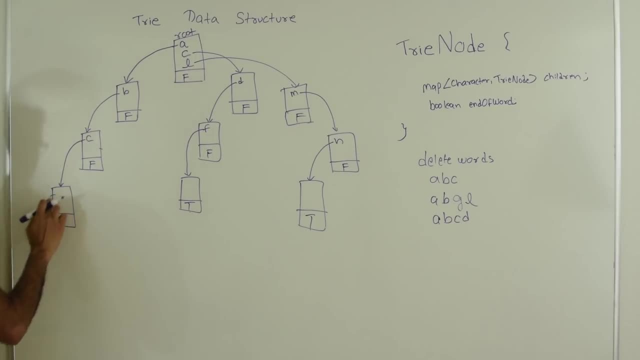 it and then go one level up and delete this character- and now this is empty, so we can delete it. and reach one level up and remove c here and now c is empty, so we can delete this. and similarly, now b will be removed and now b is empty, so we can also delete this. 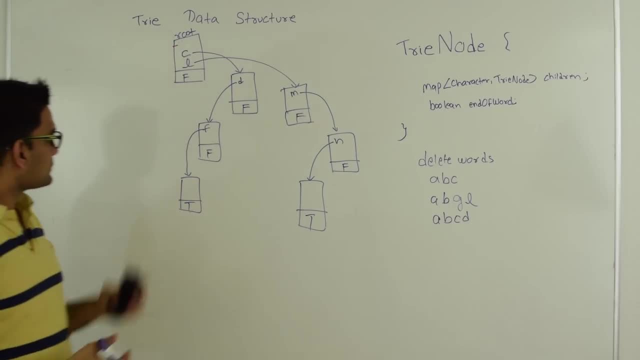 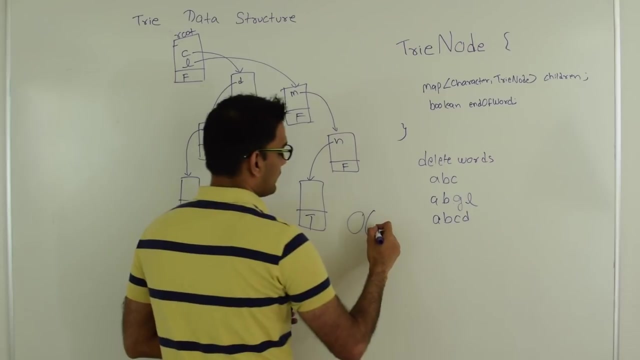 and remove a from here. So in this way, we deleted all the words, all the three words, from this trial. Again, the time complexity will be: if average length is l and all the words are this number of words are n, then l into n will be the time complexity for deletion. 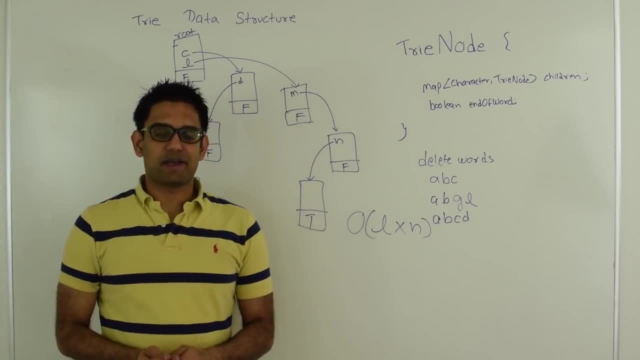 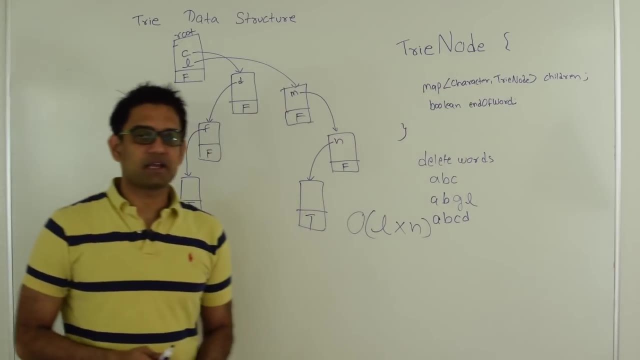 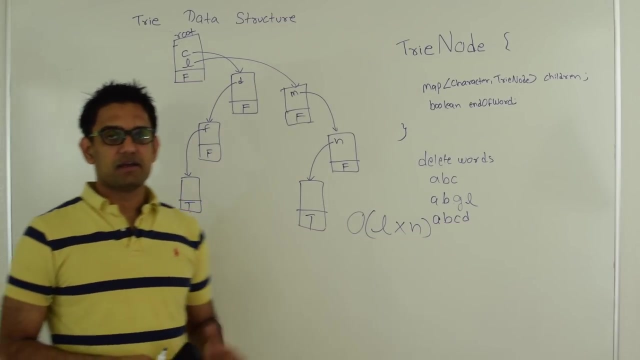 So this is all I have to talk about trying. There are tons and tons of applications of trial like doing prefix based searching. If this, if the values in this map can be values of characters map can be stored in a sorted format, then we can also sort this entire try lexicographically and in general there are. 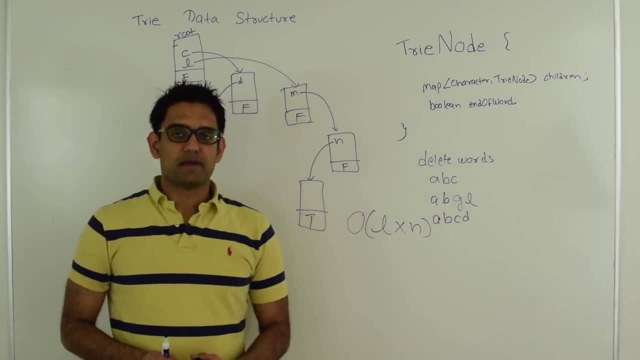 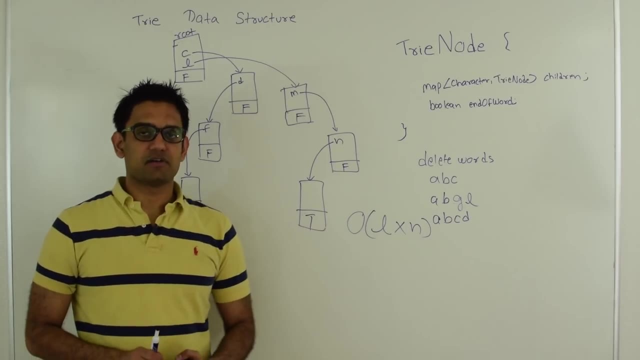 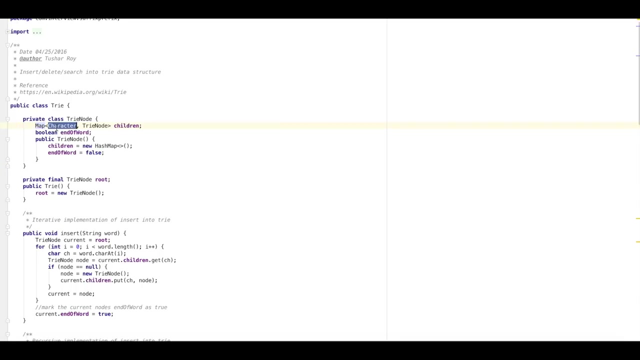 many, many applications which use try node, and probably we can discuss that in another video. So next let's look at the code implementation for try data structure. This is the try node we talked about before. So this is- this is a map With a character and try node and then end of the word. 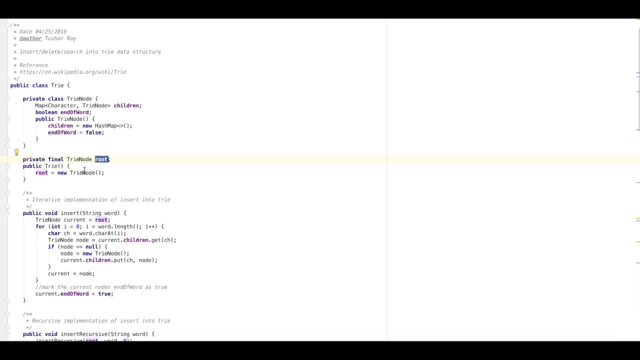 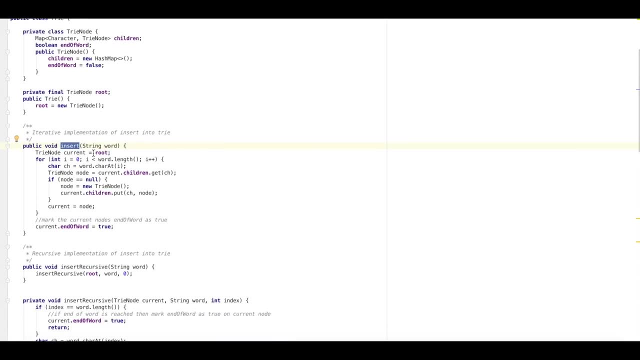 So first thing we do is we initialize our root in the constructor of try. Then we're going to do insert. So this is the iterative version of the insert and we're trying to insert a word into the try. So first our current becomes root, then we iterate through characters, one at a time, in. 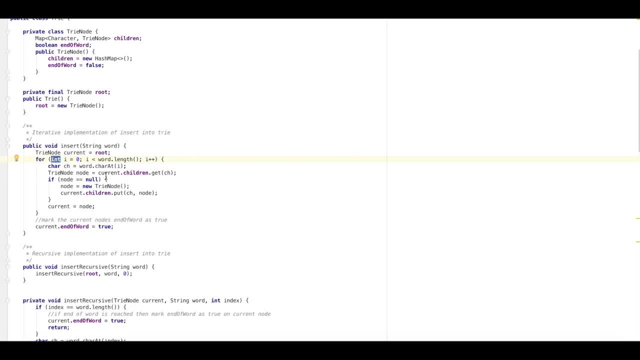 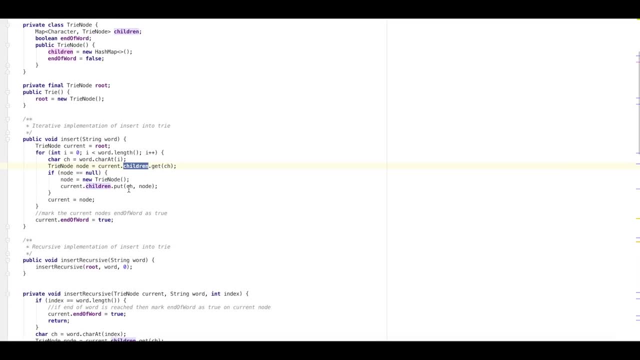 the word. And then we tried which see if current. current has This character in its map. so children is nothing but this map. So we check if current has character in the map. if it does, If it does not, so if in that case node will be null, then we create a new try node and 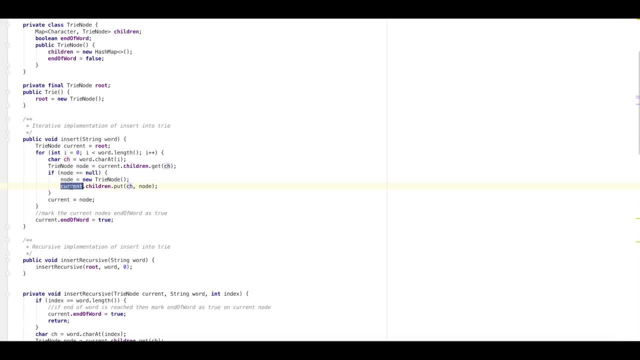 put this node and this character into the, into the currents map, and then we set current is equal to node and we keep doing it till we have characters in the word and in the end we just mark currents, end of word, as true, as we discussed before in the video. 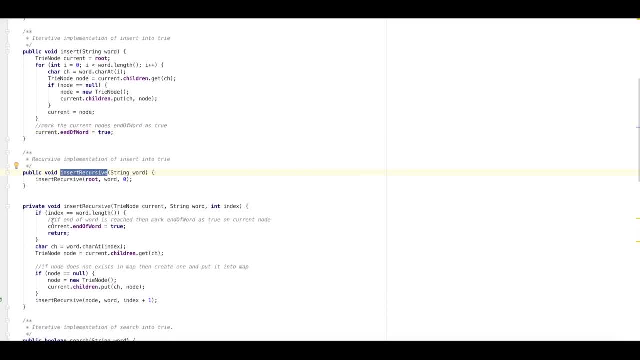 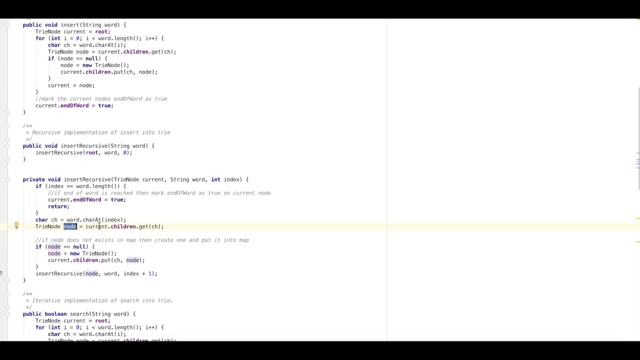 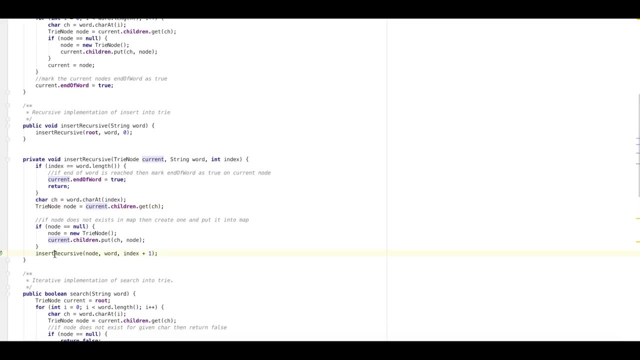 and then there is the recursive version, which is pretty much doing the same thing as in the iterative version: getting the getting the node for the currents from the current children and then checking if it is null. if it is, then putting into the map and then calling insert recursive. recursive function again. 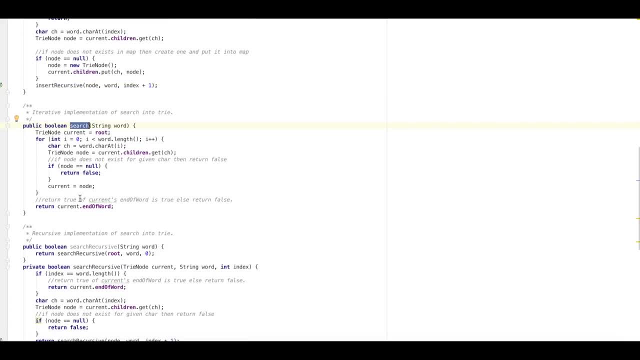 Let's look at the search. Search also is search iterative and search recursive and search iterative: We are looking if this word exists in this try or not. So again, current becomes root. again I tried through all the characters in the word. then we get the node for the currents chill from the currents map, which check if this character. 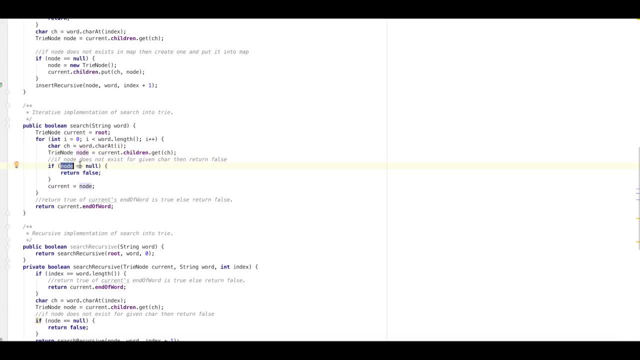 exists or not. If this node does not is null, that it means that this character doesn't exist in a map, and then we instantly return false. Otherwise, current becomes node And in the end we just return currents, end of word. So if this, if this word exists in the map, then this current end of word should be true. 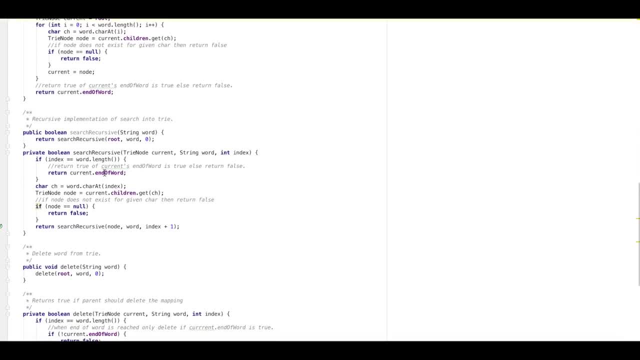 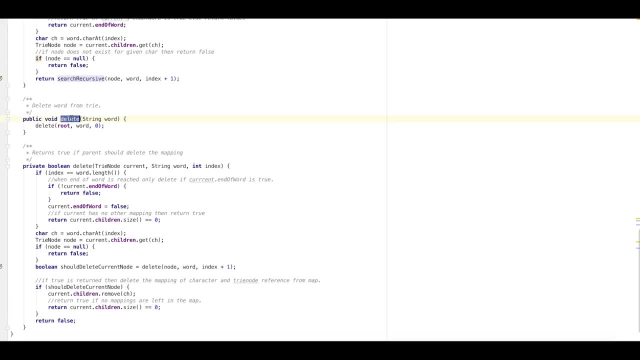 for this word to exist in the try and similarly, the recursive version is exactly same as the iterative version. and finally we have delete. So we are trying to delete this entire word. So this is the recursive version. So we first call delete with root word and index 0. 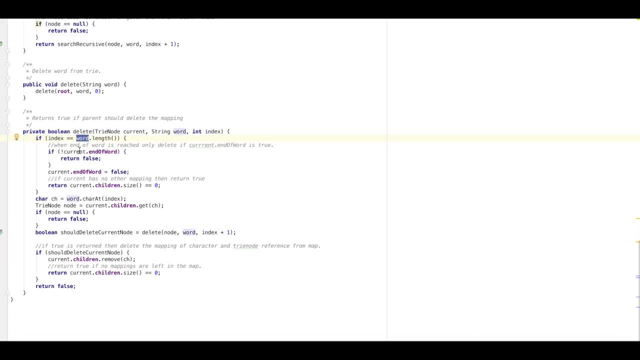 So we check if index It has reached the word length. if it has, then we check if current is end of word. if current is not end of word, it means that this word does not exist in the try and will not delete anything. So we return false. otherwise we set current end of word as false and then we return if. 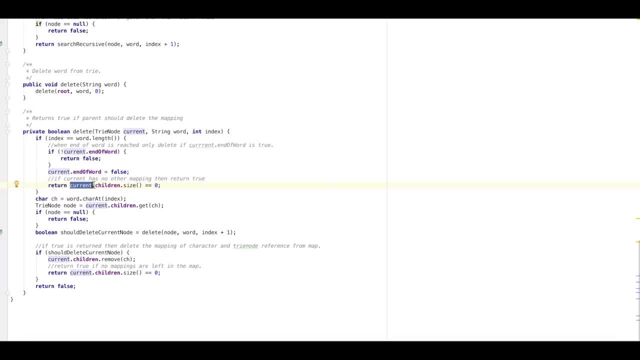 we return true if the current currents map is empty. otherwise return false. and this we are returning to give an indication to the calling function That they can delete this reference from their map. So this is the. this is if we reach. index is word length. 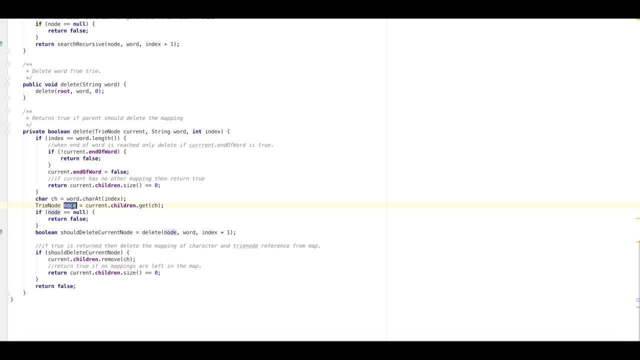 Otherwise we get the character and then we get the node for that character from the map. if node is null, it means that this word, it does not exist in the dictionary. the word we are trying to delete does not exist in the dictionary. So we instead return false. otherwise we call this recursively and should delete current.